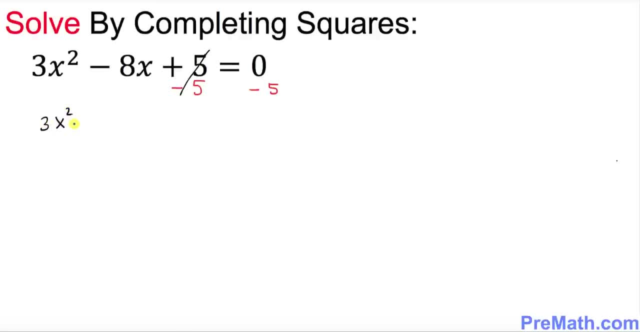 So we got 3x squared. minus 8x turns out to be equal to negative 5.. So the next thing, what we need to do is we must make sure that our leading coefficient must be 1.. Now it is 3, so the only way we can do it make it 1 by dividing by 3.. If you want to divide this one by 3, you must divide across. 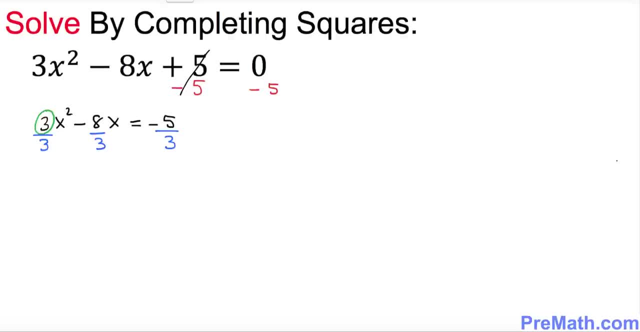 the board. So far, so good. So what we got over here is: 3 over 3 becomes simply 1x squared minus 8 over 3x equals to negative 5 over 3.. So the next step is: I want you to just look at the coefficient of x. So just look at 8 over 3.. Don't worry about this. 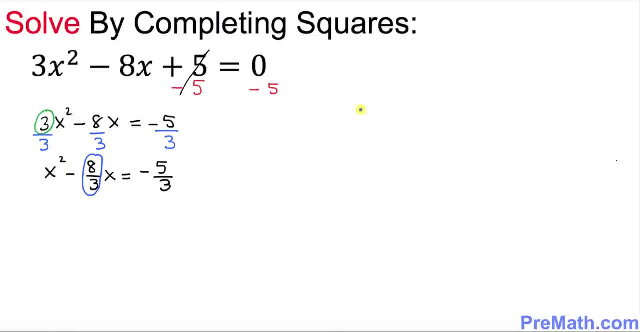 negative sign. Whatever this sign, ignore it. So I want you to just put down 8 over 3 right up here. I want you to divide this one by 2.. Dividing by 2 is same as multiplying by 1 over 2.. So far, so good. So let's go ahead and multiply 8 times 8 is 8 times 1 is 8 divided by, at the bottom, 3 times 2.. 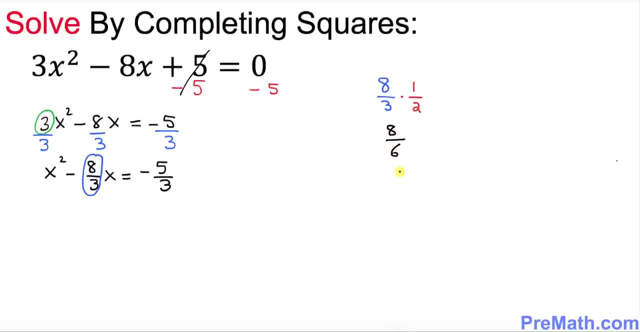 is 6, and if you reduce it that becomes 4 over 3. so far, so good. and now, whatever you got this one, I want you to square this one. so, whatever we got this quantity 4 over 3 squared, we're going to add on the both side of these equations. so that's, let's go ahead and do that one. so I'm going to. 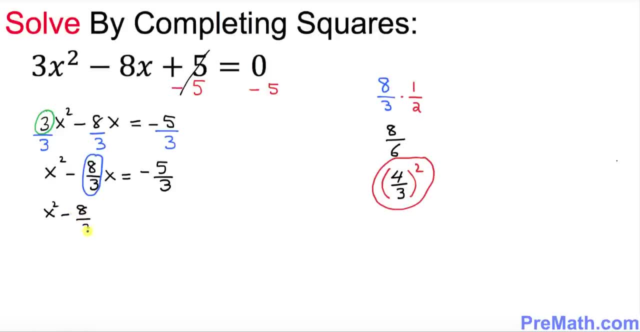 put down x squared minus, 8 over 3 x. and then I want you to put down plus equal to negative, 5 over 3 plus. now let's go ahead and add this quantity: 4 over 3 squared on both sides. so far, so good. 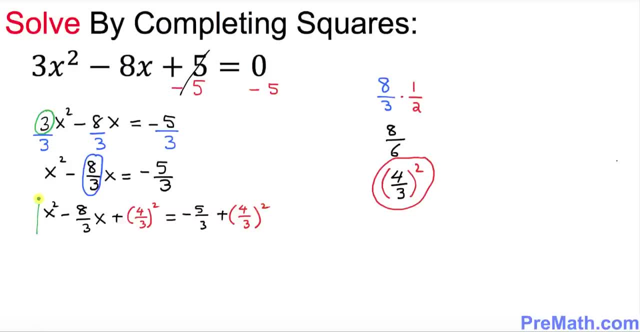 now I want you to just focus on the left hand side on this box. this represents a complete square of x minus 4 over 3 squared. now you might be wondering: how did I get that one? well, this x showed up right up here, this 4 over 3. 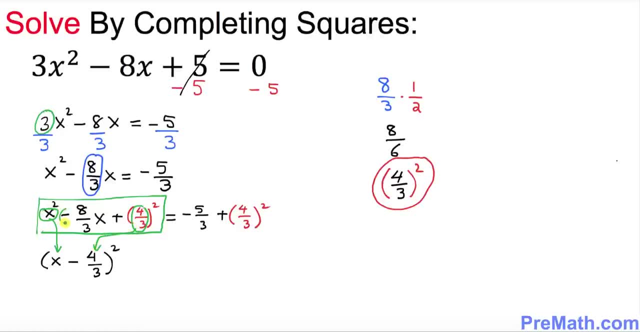 just came over here and this negative sign, whatever you see, this is in the middle. whatever this sign equals to negative 5 over 3, and then this is could be written as 16 over 9. so far, so good. now the next thing, what we're going to do. 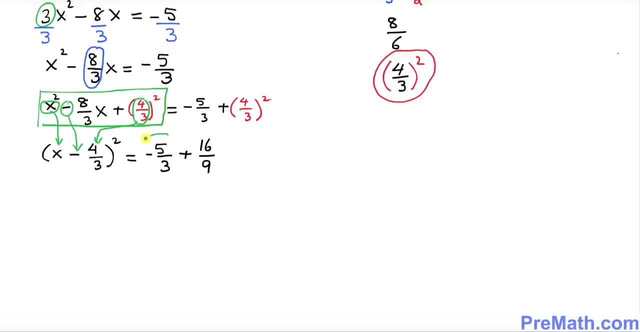 is. I want you to just go ahead and write down this part somewhere here, so I put these fractions right up here, as you can see now. you see the denominators are 3 and 9. we want to make the same denominator, so I can divide this one, the first fraction, by 3. I'm going to multiply and. 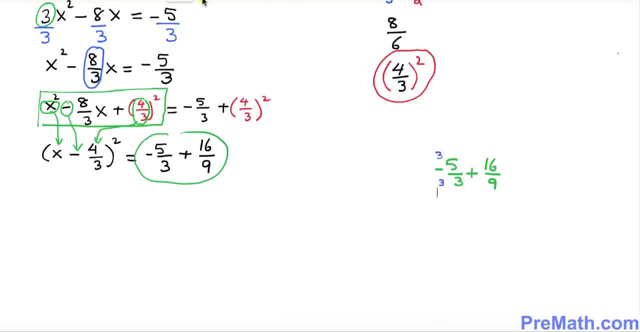 divide by 3. so that's going to give us negative 5 over 3. so that's going to give us negative 15 over 9. so far so good. so negative 5 over 3 is same as negative 15 over 9 plus 16 over 9. and since we have 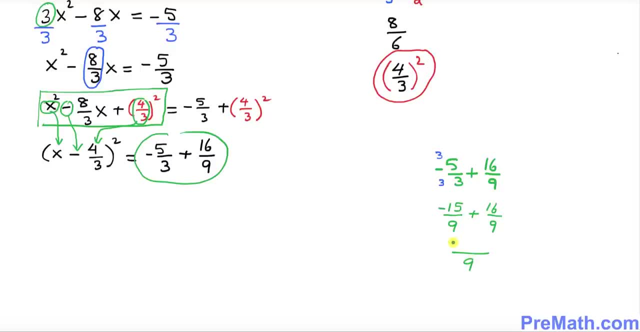 the same denominator to 9, so we got negative 15 plus 16. this turns out to be 1 over 9. so that means this right hand side structure is going to 자 is same as 1 over 9, and on the left-hand side we have X minus 4 over 3 square now. 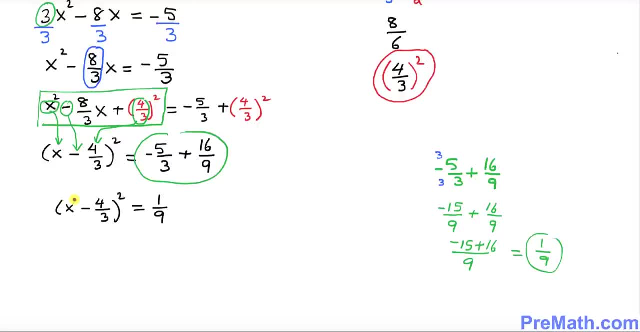 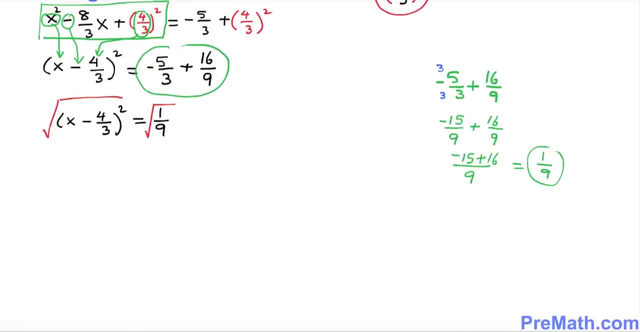 we want to solve for X, so we're going to want to remove this square. how you can undo this square? by taking the square root on both sides. so far, so good. so the next step, what we're going to do, is so you can see this square and square root.